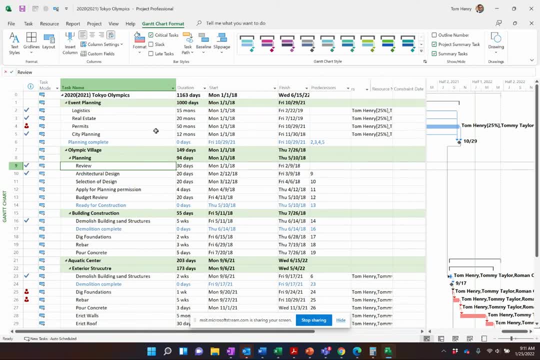 Hi there, In this video I'm going to show you how to build out your work breakdown structure within Microsoft Project. So you can see this is a pretty complex project schedule I've put together. I've used this in some of my previous examples. You can see that we have all of my 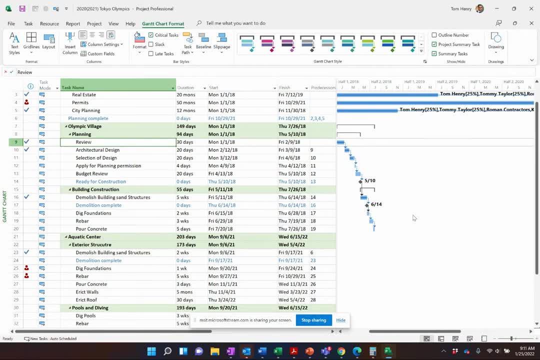 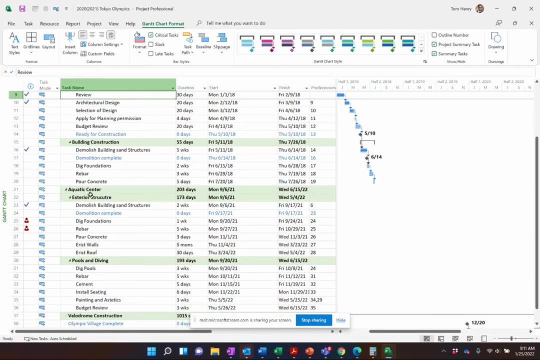 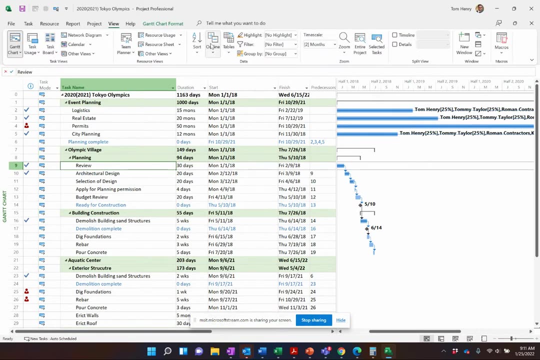 different tasks. They are linked together. We have logical dependencies between the tasks and we have a structure within the schedule, whether that be a selection of summary tasks and tasks, milestones, et cetera. What I can actually do is come in here and take a look at. 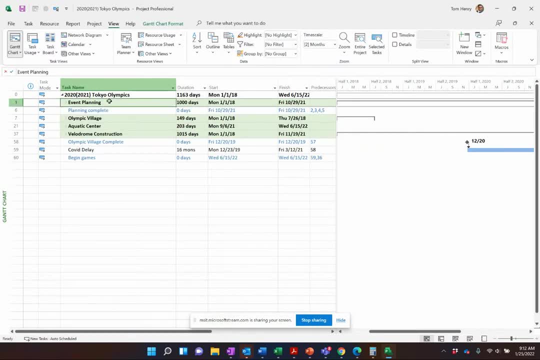 my outline levels and go down to level one which kind of shows me high level, my summary tasks or phases within the project and some milestones here as well. That's, the beauty of using summary tasks is the fact that you can indent the task beneath them and then have different levels and 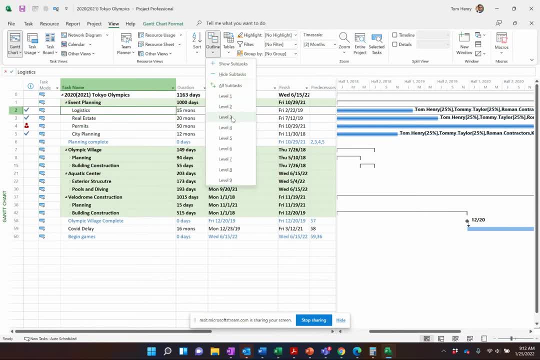 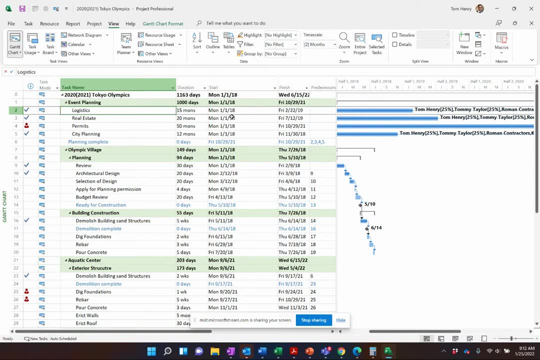 I can drill in, And if there's a level below that I go to outline level three, et cetera. So you can drill into your project and drill out of your project. Now a lot of people will name their tasks one, 1.2,, 1.3. Obviously, that becomes a nightmare when you add a new task and you've 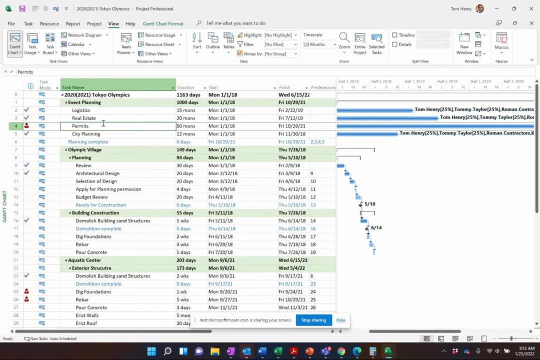 got to go through and rename everything. So that's not the way to build out your work breakdown structure. In fact, Microsoft Project makes this available to you in two different ways. Let me show you. So if you go to any Gantt chart, view this, I can go to the Gantt chart format And in 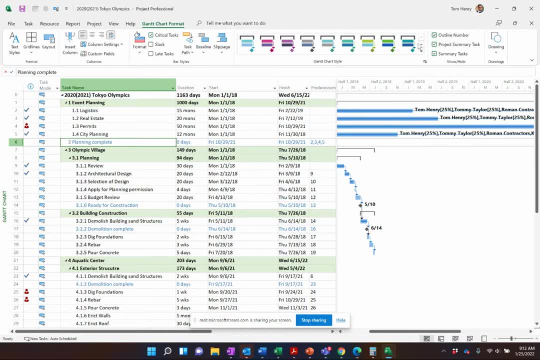 here I can check this outline number. What this does is it pulls into the name of my task the work breakdown structure One: 1.1, 1.2,, 2, 3, 3, 3.1, 3.1.1, et cetera, So on and so forth. It really helps you. 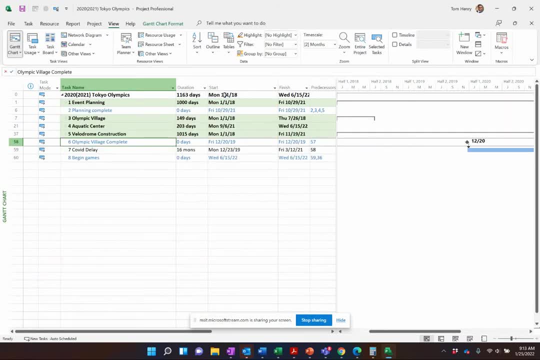 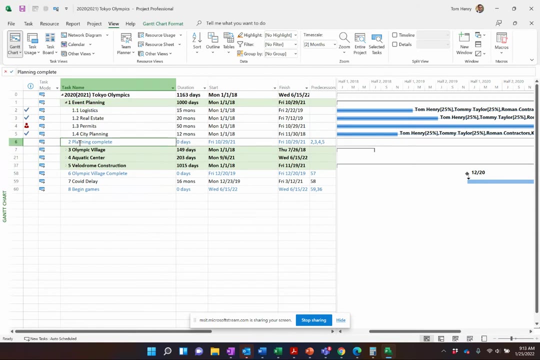 to. when you're drilling in and out, right back to level one, you can see phases of my project. What you will notice is that, Because this milestone is at the same level as my summary task, it will have that same outline number, level of indentation. 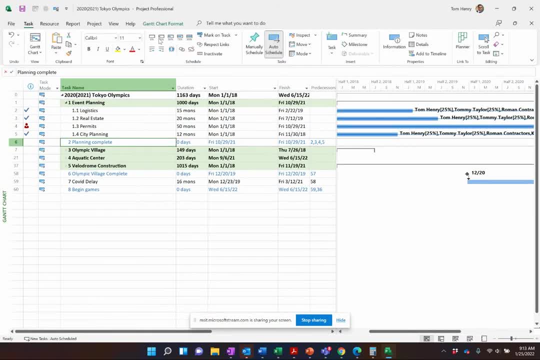 So if you don't like that, what you can do is indent that particular milestone like so: Now it becomes at the same level as level one and that kind of goes away. So now this becomes two, three, four, et cetera.